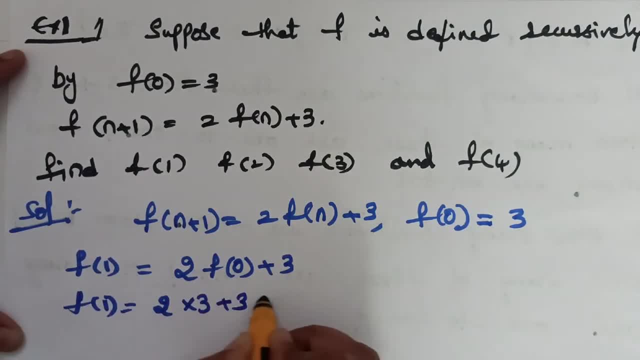 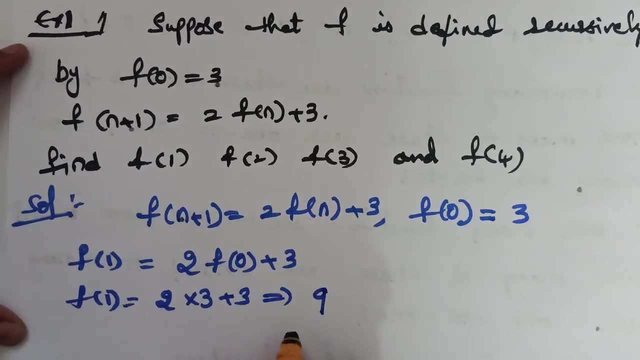 where f of 0 is 3, 2 into 3 plus 3 implies 2 into 3 is 6 plus 3 is 9, therefore f of 1 is 9, f of 2,. this is equal to: by substituting: n is equal to 1, 1 plus 1 is 2, this is equal to 2. 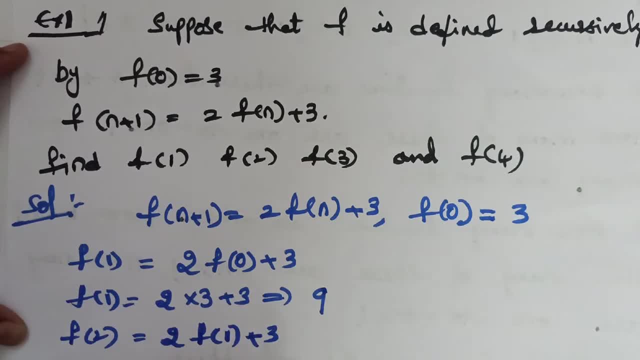 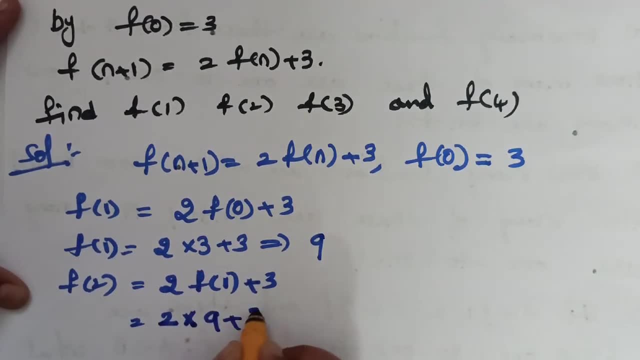 into f of 1 plus 3, this is equal to 2 into. just now we calculated f of 1,, that is, 9,. 2 into 9 plus 3,. 2 into 9 is 18 plus 3 is equal to 21,, and f of 3,. 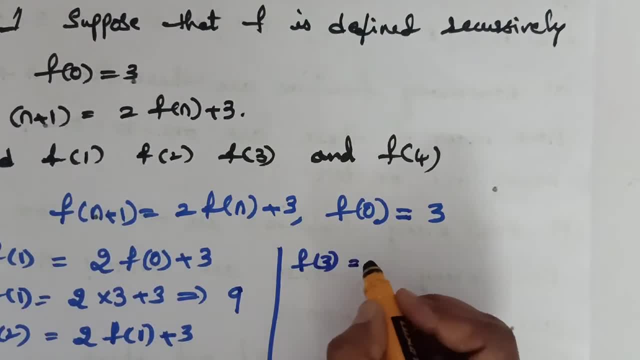 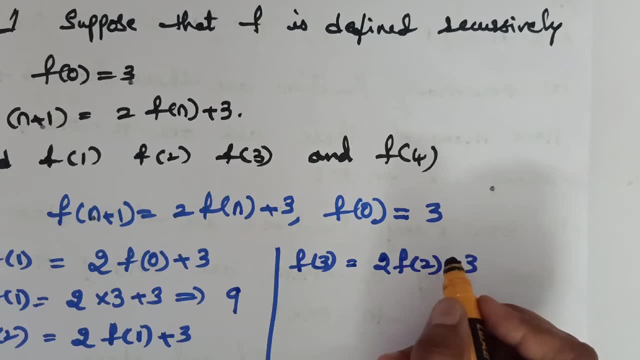 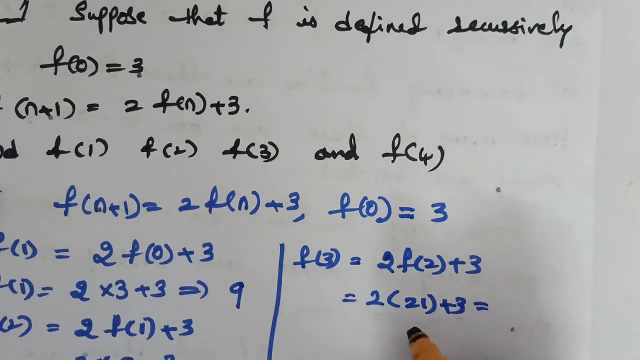 f of 3 is equal to 2 into f of 2 plus 3, by substituting n is equal to 2, we get this f of 3 value. so this is equal to 2 into 21 plus 3 is equal to 2 into 21,. 21 into 2 is 2,. 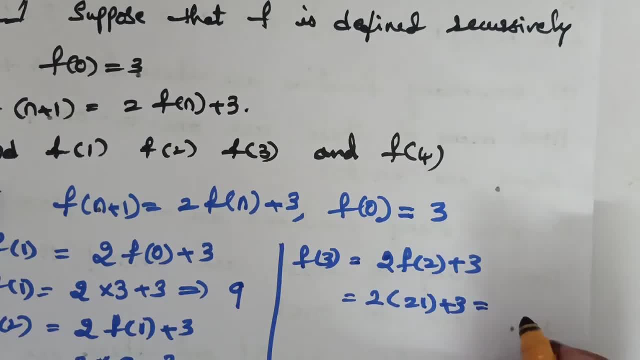 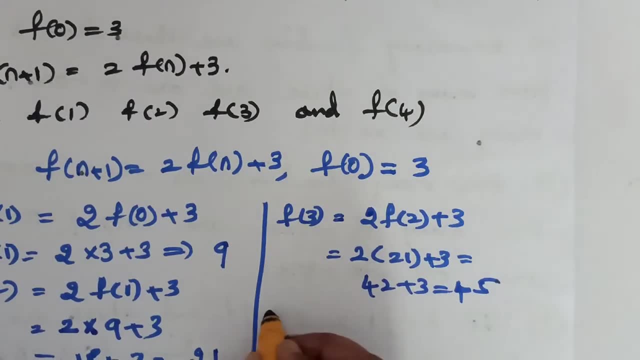 2 is a 2, 1 is a 2, 2, 2 is a 4, 42,. 42 plus 3, is equal to 45, so f of 3 value is 45,. similarly, find out f of 4, f of 4 is 2- into f of 3 plus 3,. 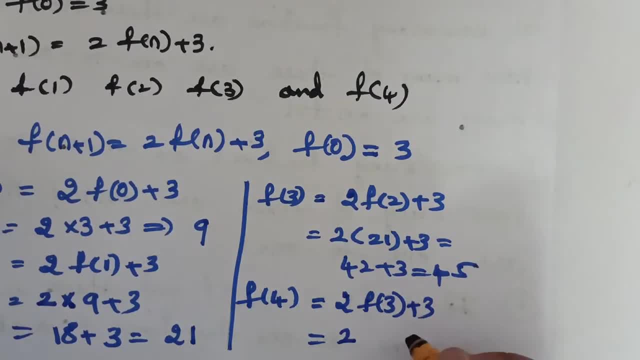 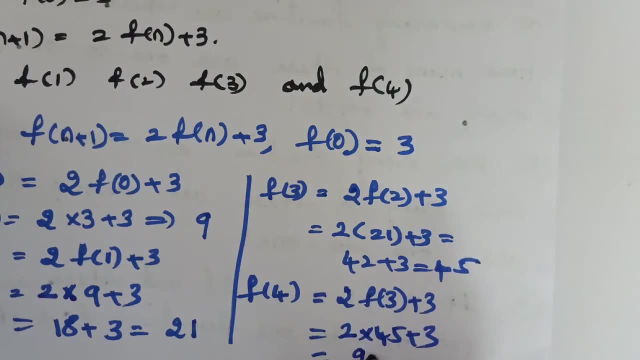 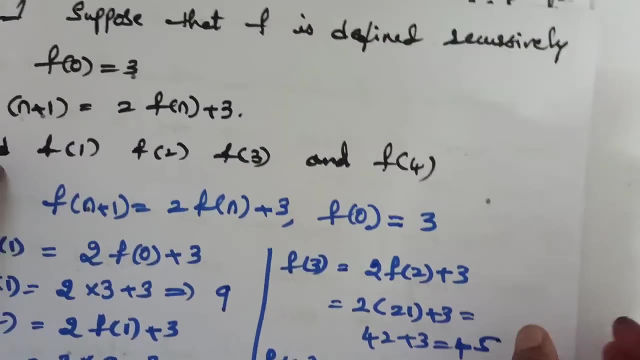 this is equal to 2 into where f of 3 is 45 plus 3, 45 into 2 is 90, 90 plus 3 is equal to 93,. okay, this is about first problem. let me explain once again. suppose that f is defined recursively. 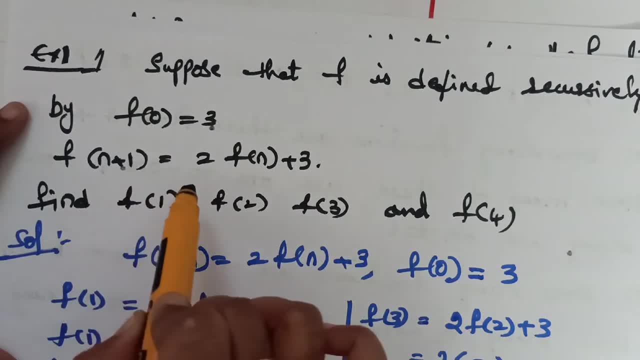 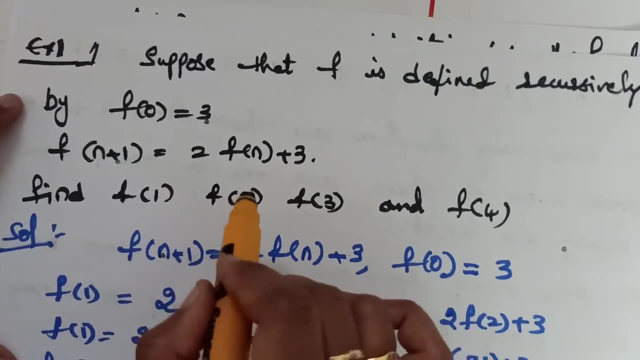 by f of 0 is 3, f of n plus 1 is equal to 2. into f of n plus 3, find f of 1, f of 2, f of 3 and f of 4, here you have a recursively defined function, that is, f of n plus 1 is equal to 2, into f of n. 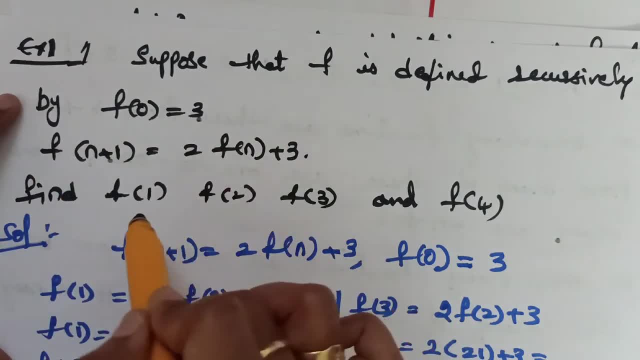 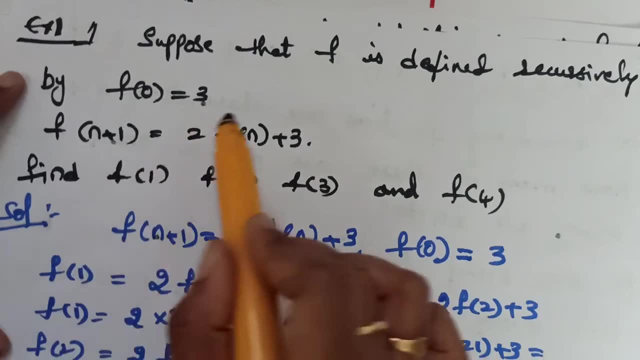 plus 3,. using this recursive defined function, you need to find out f of 1,, f of 2,, f of 3,, f of 4,. okay, to get f of 1, you need to substitute n equal to 0, by substituting, n is equal to 0,. 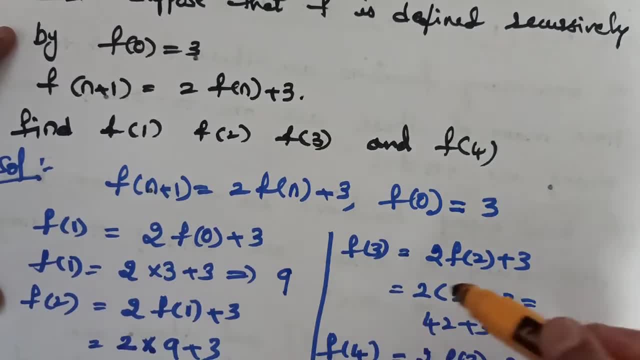 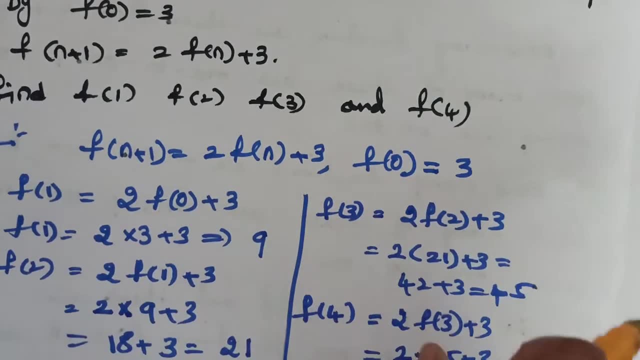 we got f of 1,. by substituting n equal to 1, we got f of 2, by substituting n equal to 2, we got f of 3, and by substituting n equal to 3,, we got f of 4,. so these are the f of 1, f of 2,. 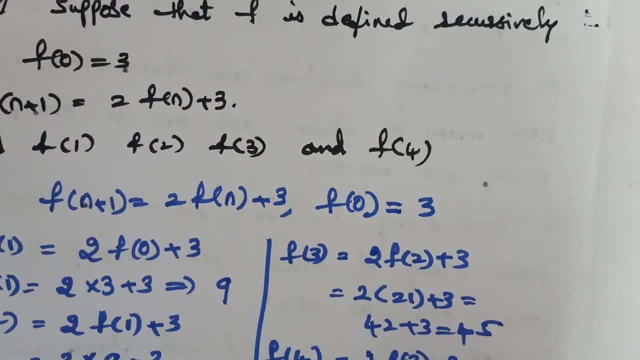 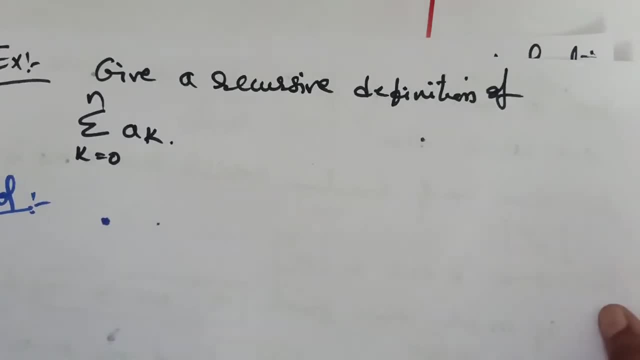 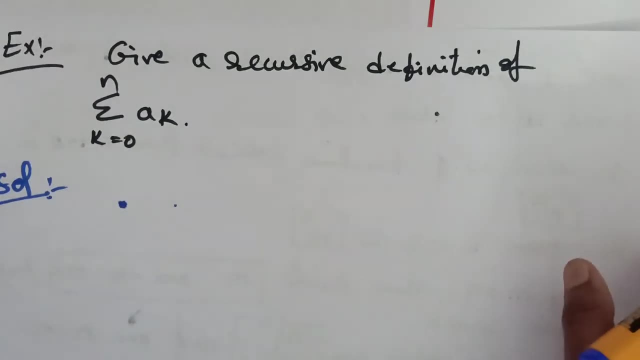 f of 3, f of 4 values. okay, this is about first problem. okay, next second problem: give a recursive definition of summation. k is equal to 0 to n a k. okay, you can identify the difference to the last problem. 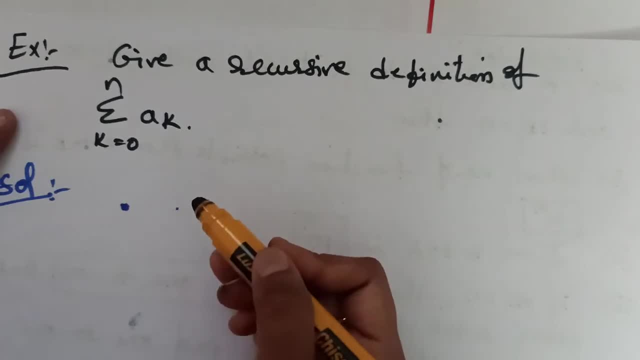 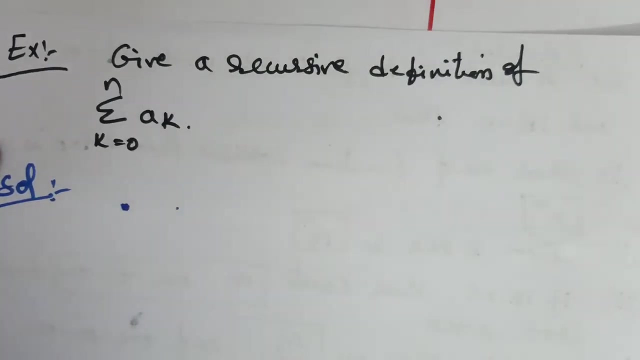 in this problem. in the last problem we had a recursive definition, so using this definition we calculated other values. but here to this you need to find out a recursive definition of this summation. k equal to 0 to n, a k recursive. just now we discussed in a 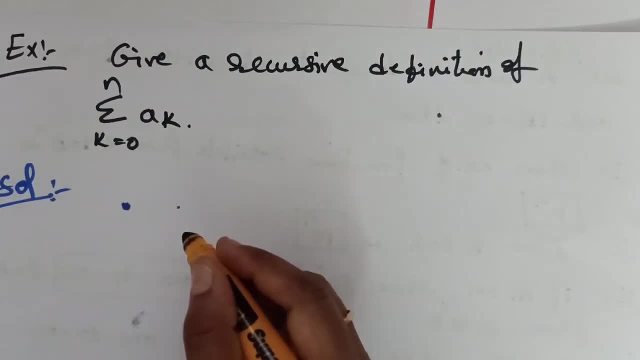 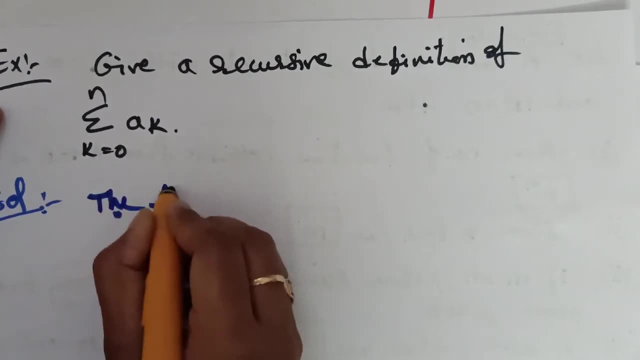 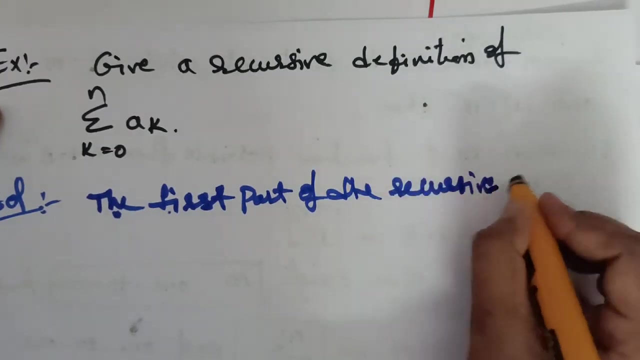 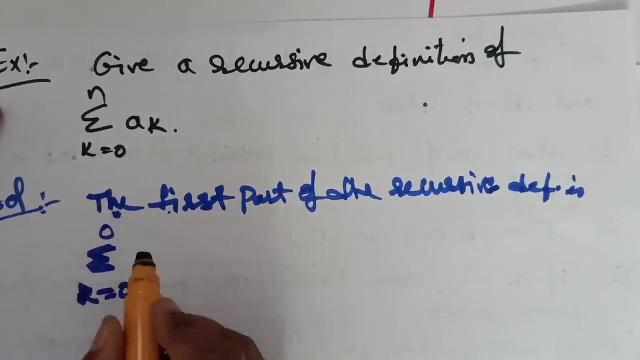 formula that is in the definition. this contains two steps. okay, solution, the first part of the recursive definition. the first part of the recursive definition is summation k equal to 0 to 0, by substituting n equal to 0, in the basis step. you need to: 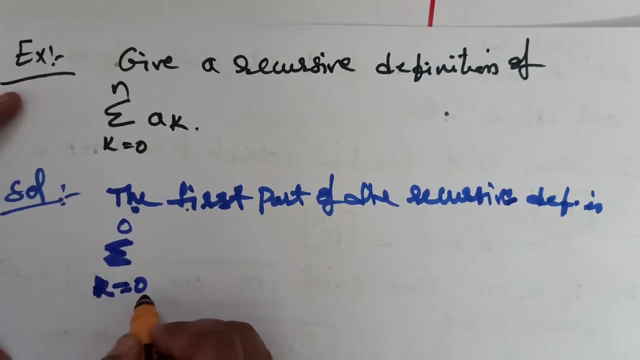 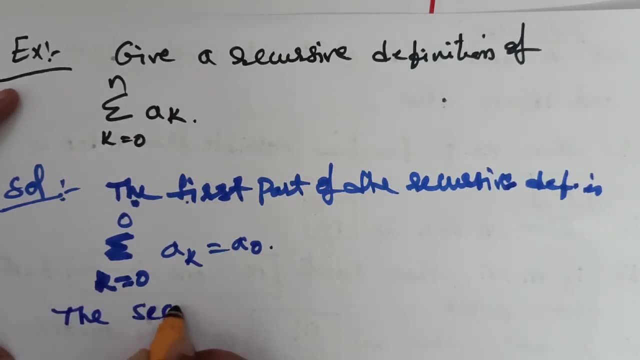 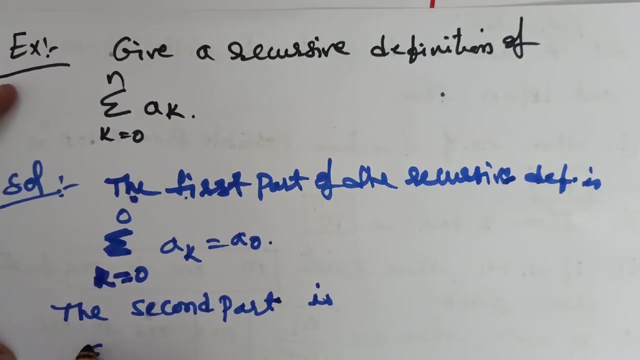 substitute n equal to 0, summation k is equal to 0 to 0,. a k is equal to a 0,. the second part contains: summation k is equal to 0 to n plus 1, a k is equal to. by expanding this: 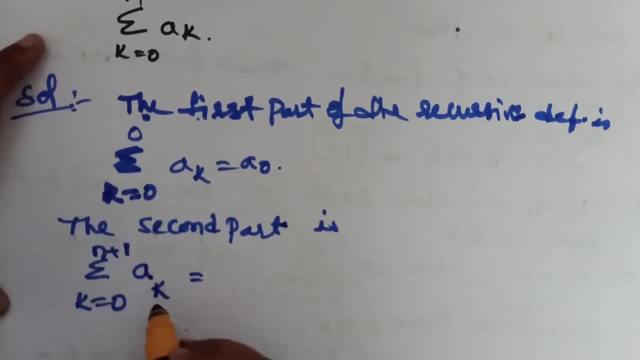 summation: k is equal to 0 to n plus 1, a k is equal to a 0 plus a 1, plus a 2, plus so on, plus a n plus a n plus 1, okay on expanding this summation. 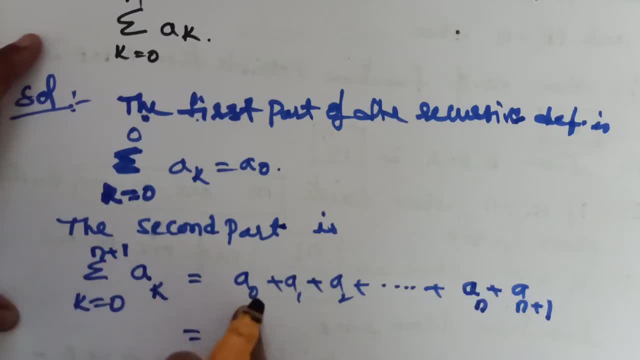 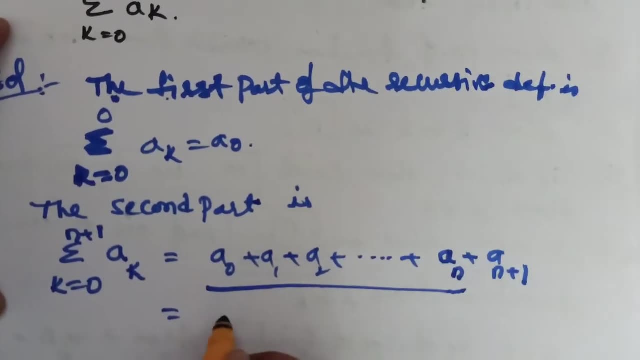 you get by taking k equal to 0 to n plus 1, you get a 0 plus a 1, plus a 2, plus so on, plus a n plus a n plus 1, so this term you can write it as summation: k is equal to 0 to n. 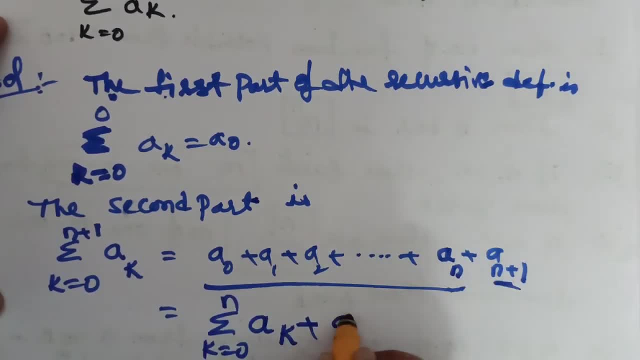 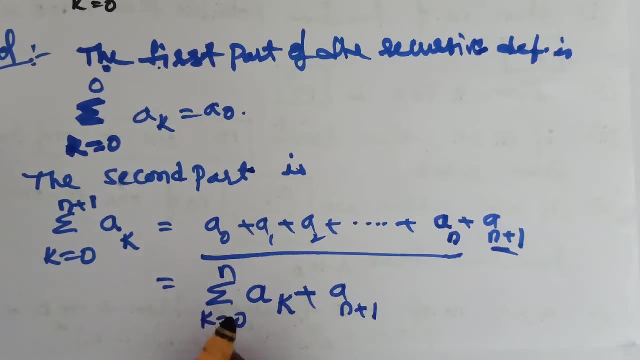 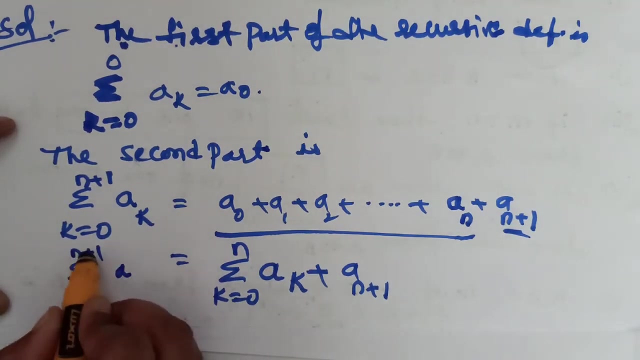 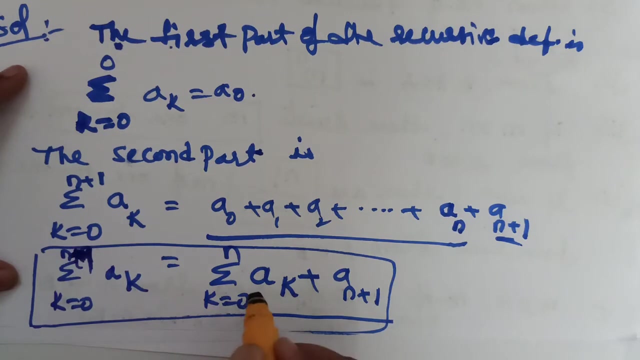 a k plus you have a n plus 1, this is about the recursive definition of summation. k is equal to 0 to n plus 1, 0 to n a k. So therefore, the recursive definition: summation k equal to 0 to n plus 1, a k is equal to summation. 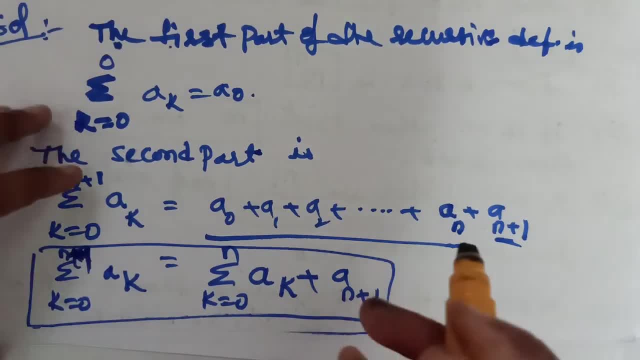 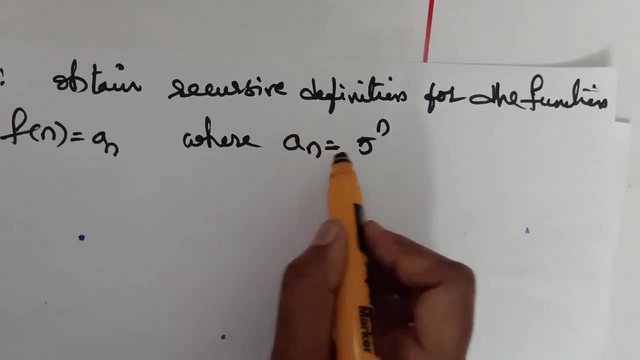 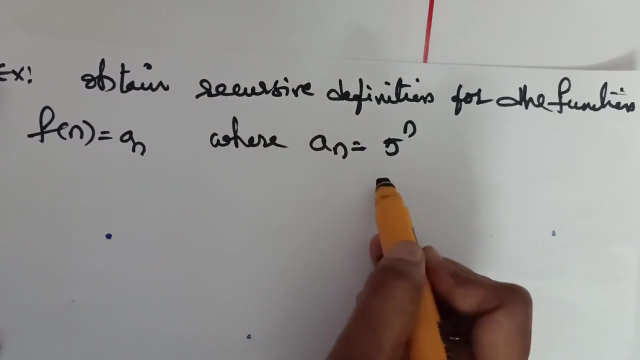 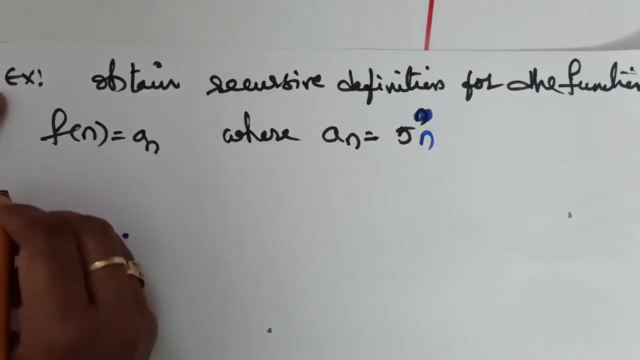 k equal to 0 to n. a k plus a n plus 1.. Okay, This is about Next third one. Obtain recursive definition for the function f of n is equal to a n, where a n is equal to 5 into sorry 5 power n, sorry 5 into n. Okay, Solution: a n is 5 into n. f of n is equal to given. 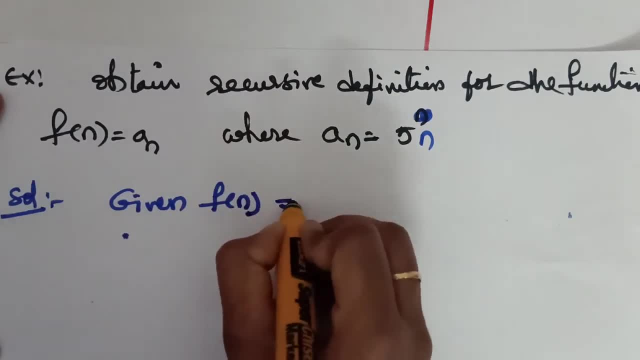 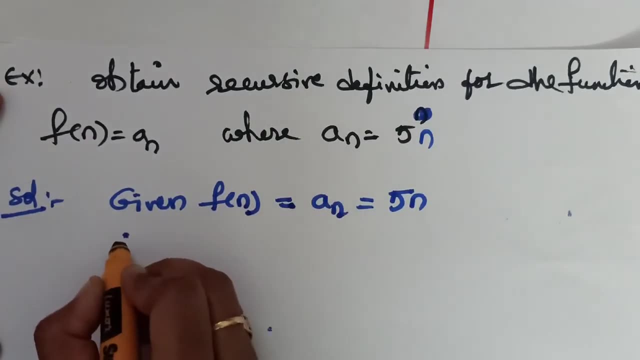 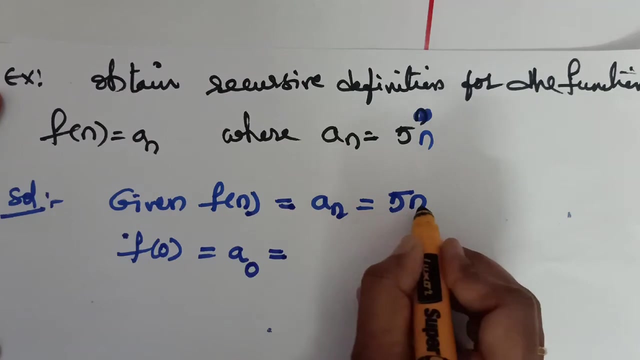 when function f of n is equal to a n, what is a n? a n is 5 into n. so when n is equal to 0, you get f of 0, which is equal to a naught. that is equal to 5 into 0 is 0. 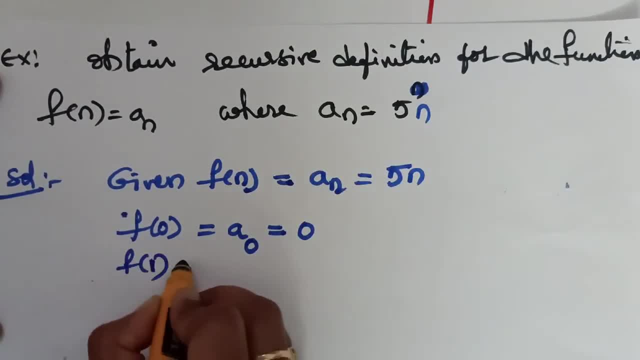 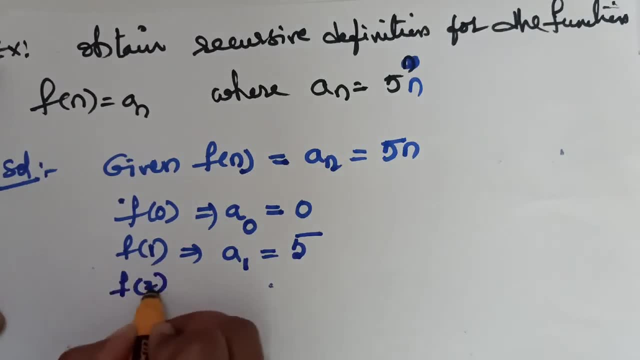 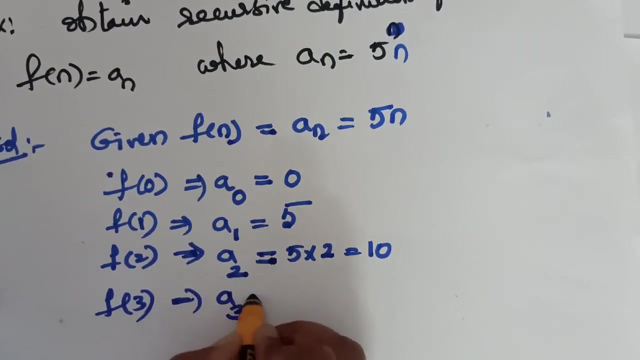 f of 1 implies a 1. a 1 is equal to 5, f of 2: this implies a 2. a 2 is equal to 5, into 2 is equal to 10, and f of 3: this implies a 3 is equal to 5 into 3, which is equal to. 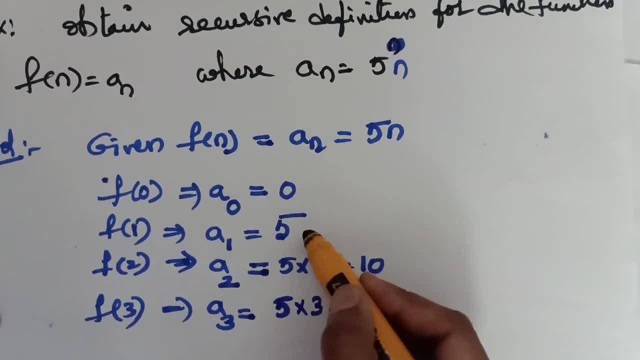 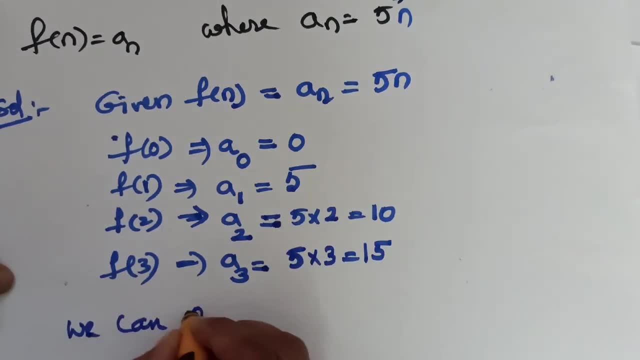 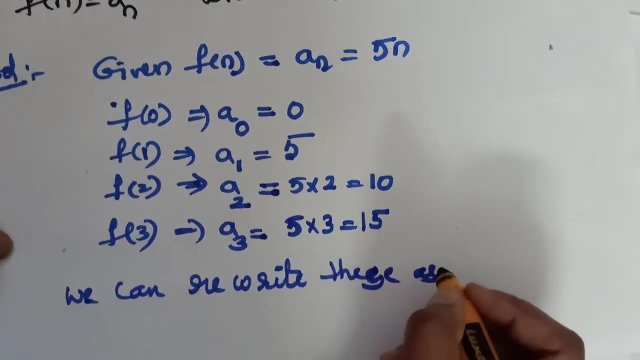 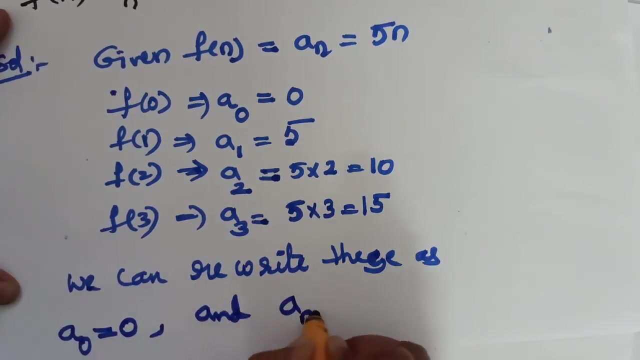 to 50.. Okay, These are A naught: A1,, A2,, A3 and so on. Okay, We can rewrite. We can rewrite these as A naught. initial condition: A naught is 0 and A? n. How can we write this? A? n as? 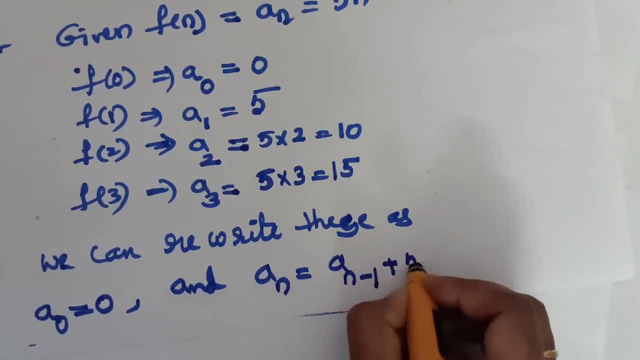 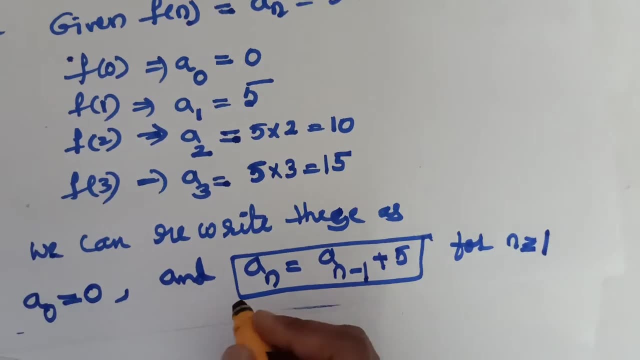 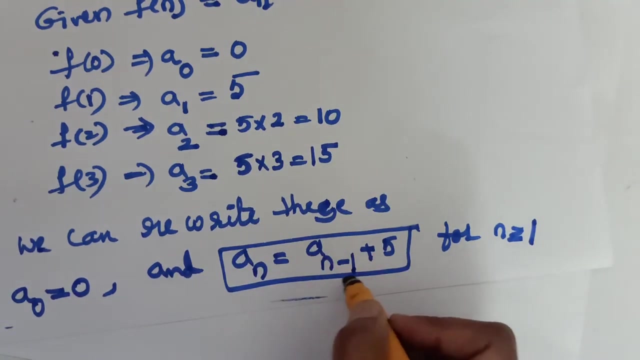 A n minus 1 plus 5 for n greater than or equal to 1.. Okay, You can write, You can rewrite these as A n is equal to A n minus 1 plus 5 for n greater than or equal to 1.. 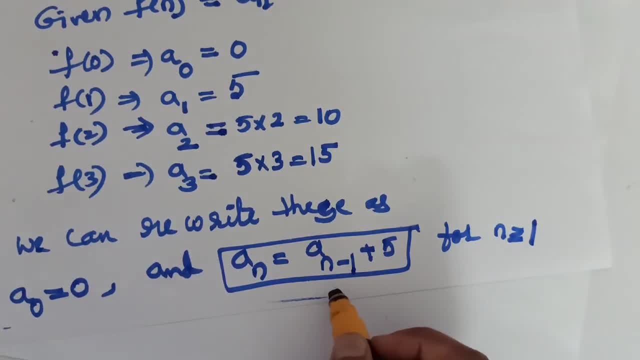 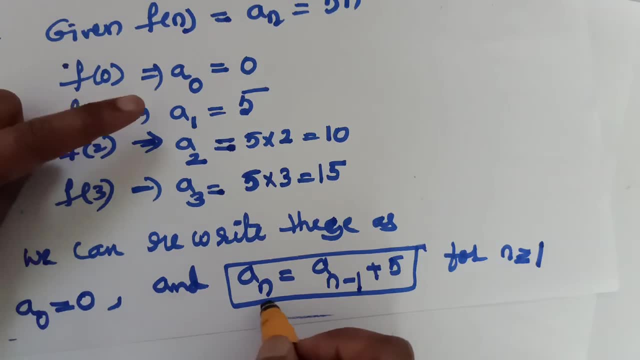 So this is a recursive definition of the given F of n. See. with this recursive definition are we getting the correct values? See, by substituting n is 0.. So we got A naught. A naught is already there. To get A1, you need to substitute A1 value. A1 is equal to. 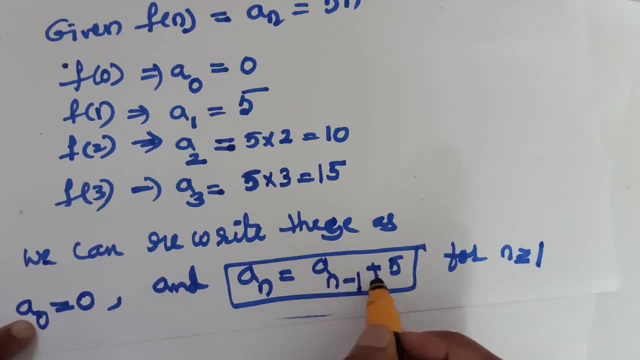 A1 minus 1, that is A naught plus 5 means A naught is 0,. 0 plus 5 is 5.. So you got A1 value. that is correct A2.. 2 is equal to A2 minus 1, that is A1.. A1 is 5.. 5 plus 5 is 10.. Next, by substituting n. 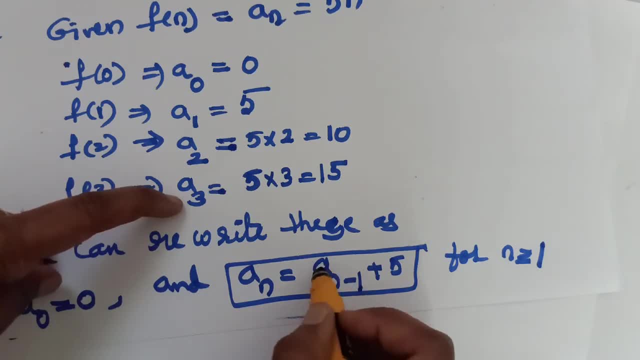 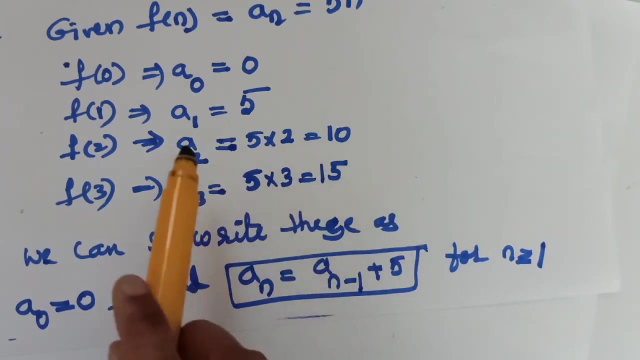 equal to 3.. A3 minus 1 is A2.. A2 is 10.. 10 plus 5 is 50. So what is A4?? A4 is 20.. A5 is 25.. By looking at this, you can easily identify. We got A1 by adding 5 to this A. 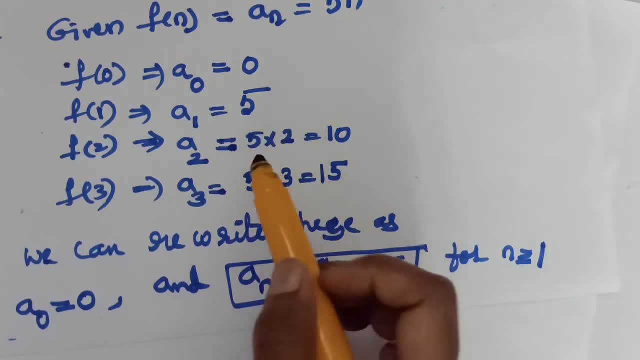 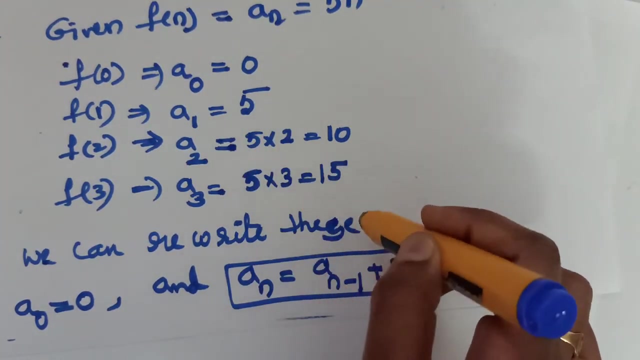 naught Next 2 times of this. that means 5 plus 5 is 10.. 10 plus 5 is 15.. 15 plus 5 is 20.. 20 plus 5 is 25.. So you can, based on that, you can rewrite. you can this as: 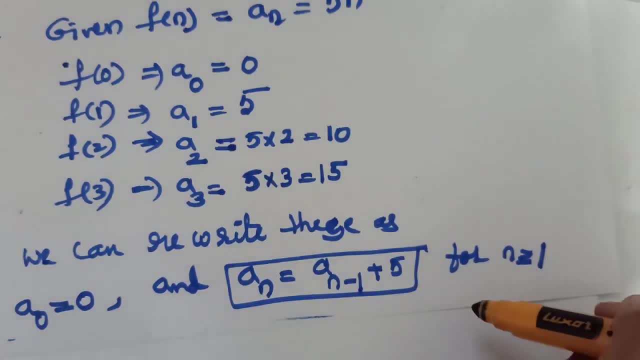 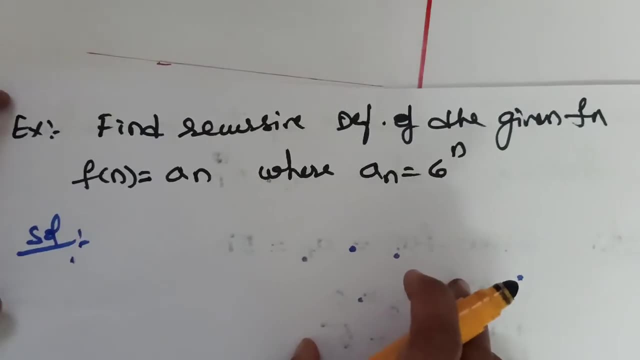 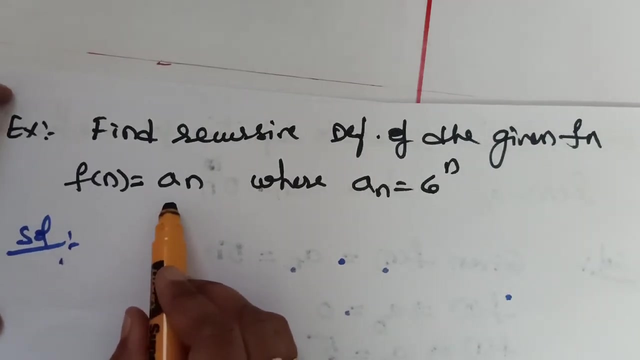 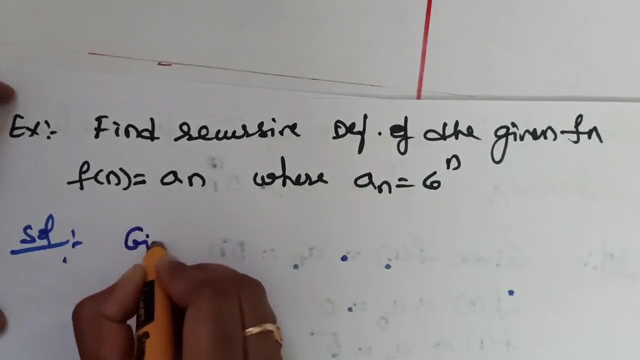 A n is equal to A n minus 1 plus 5.. This is a recursive definition for the given function F of n. Next problem: find recursive definition of the given function F of n. where F of n is equal to A n. where A n is equal to 6 power n, Here it is given. You are finding the 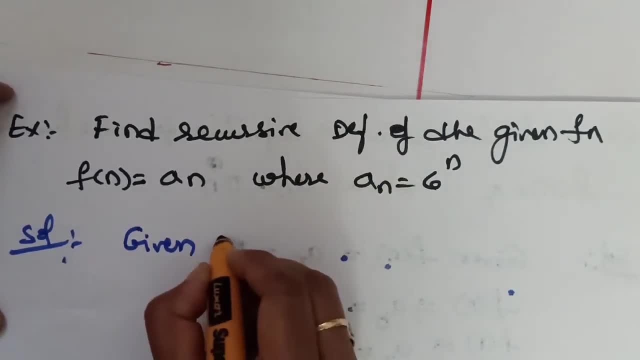 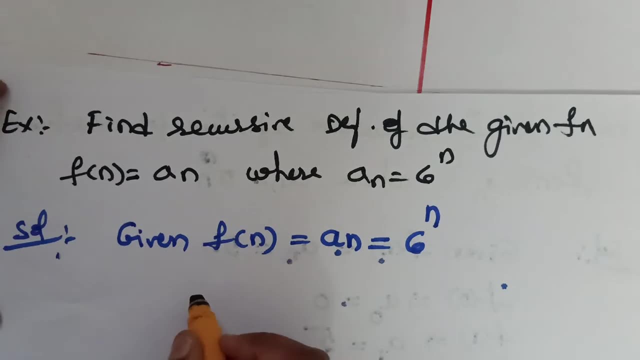 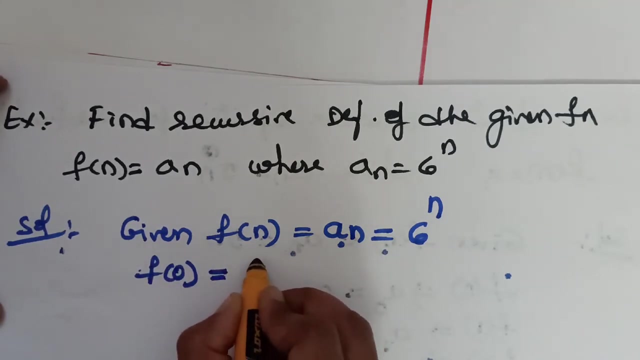 recursive definition of the given function F of n. Given function F of n is equal to A n, which is equal to 6 power n. Okay, 6 power n. So by substituting n equal to 6 power 2 where n is equal to 2.. Againruction is done also Here. it is given. You are understanding. 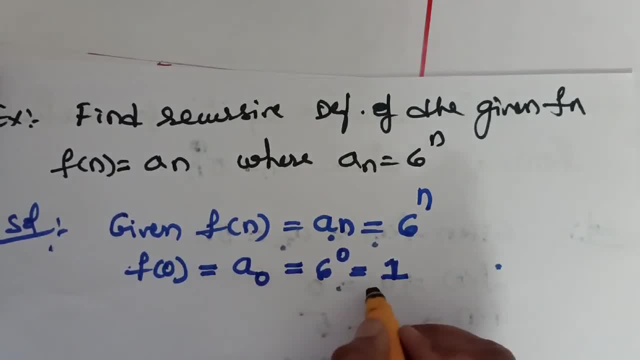 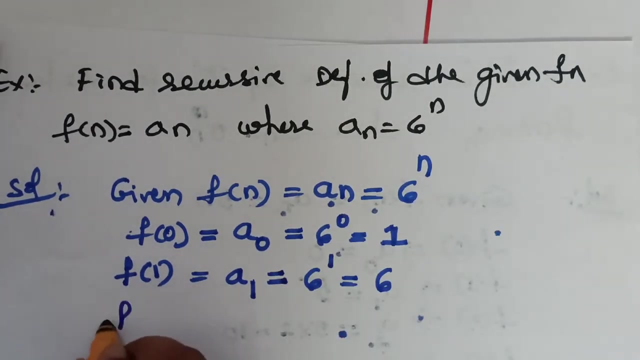 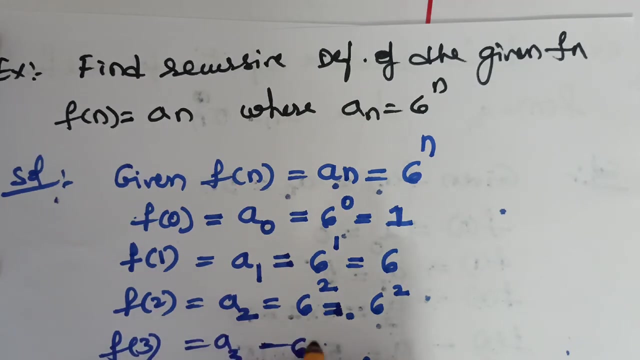 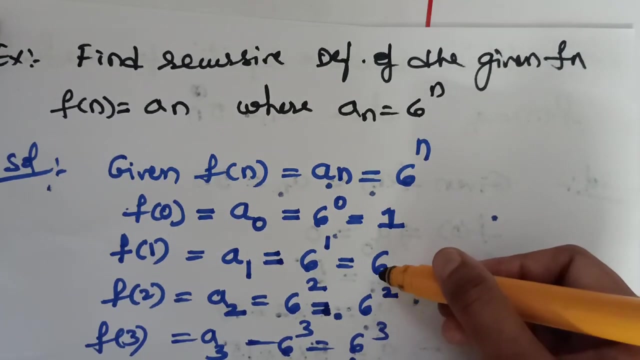 that f note of f0 is n equals to 0. Here, if it opens, you can write this as: 1 till 2 is 6 power 2, f of 3 a 3, 6 power 3, 6 power 3. if you look at these terms: f of 3, f of 2, f of 1. 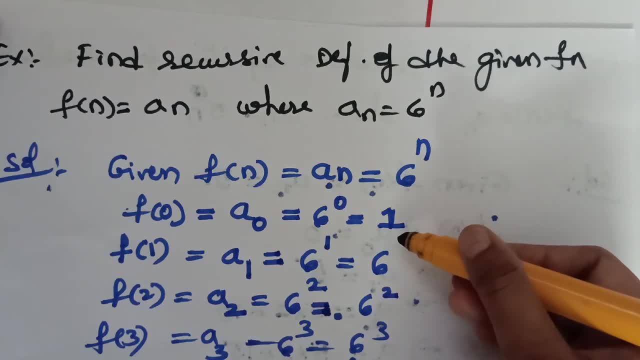 and f naught. when a naught is 1, a naught is 1. how can we find out a 1, a 2, a 3 values? ok, a 1 can be calculated by using multiplying 1 into 6. similarly, a 2 can be multiplied again. 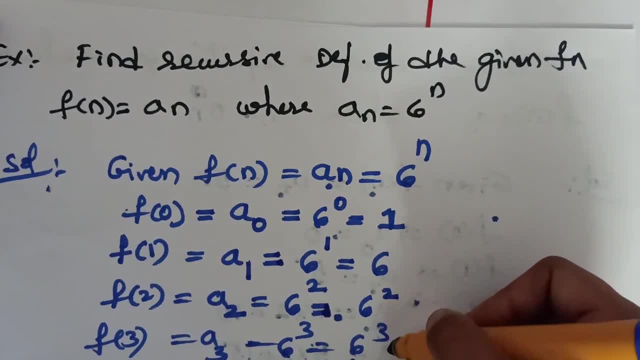 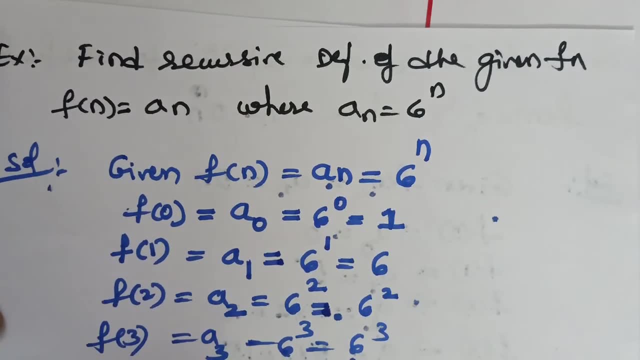 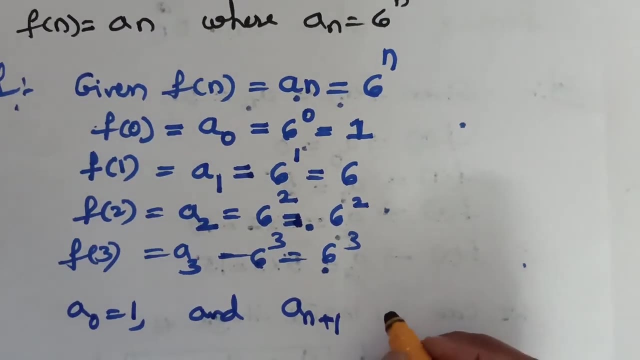 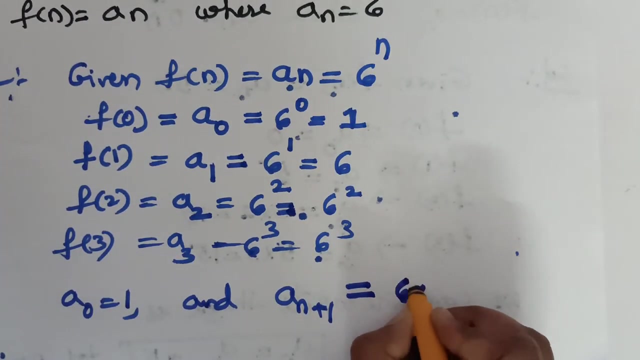 with 6 a 3. we can multiply it again with 6, so this we can write it as: because the definition can be written as: a naught is equal to 1, i a n plus 1. ok, a n plus 1 is equal to a naught is equal to 1 and a n plus 1 is equal to 6. into a n, 6 into a n. 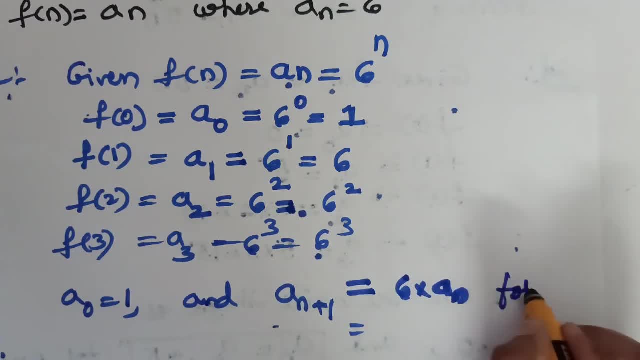 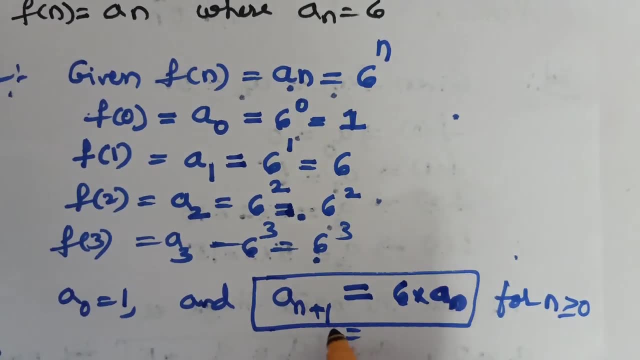 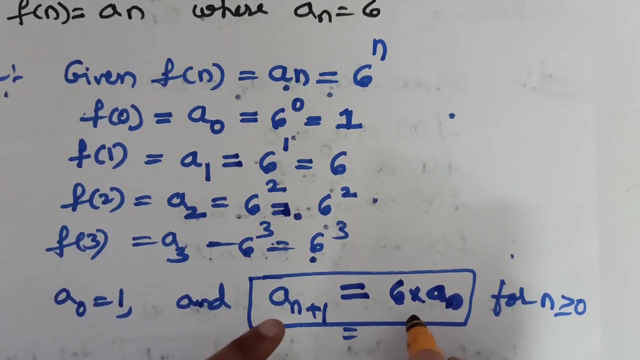 okay, this is the recursive for n greater than or equal to 0. 6 into a n for n greater than or equal to 0. so after writing this recursive definition we need to check: is it character recursive definition? yes, if i substitute n equal to 1, we get a 1, that is, 6, into a naught where a naught is. 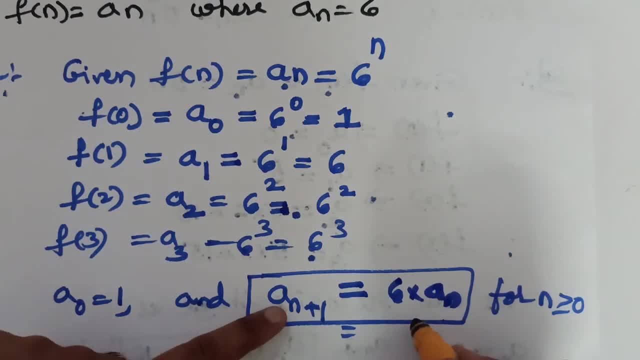 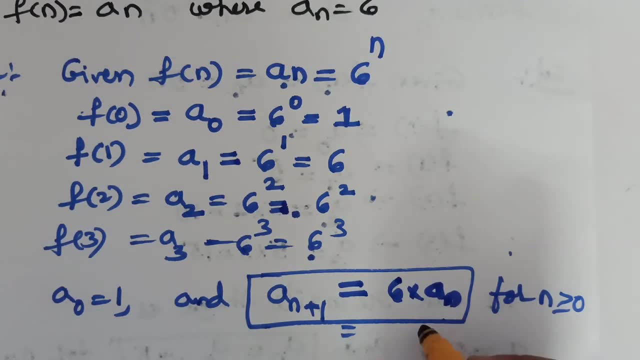 1. so 6 into 1 is 6. so when i substitute n equal to 1, you get a 2. so 6 into a 1. again, 6 into 6 is 6 is, yes, 6 power 2, 6 power 3, 6 power 4. you are getting the correct values with these. 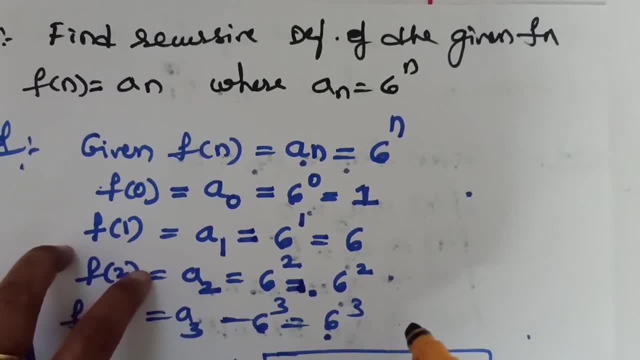 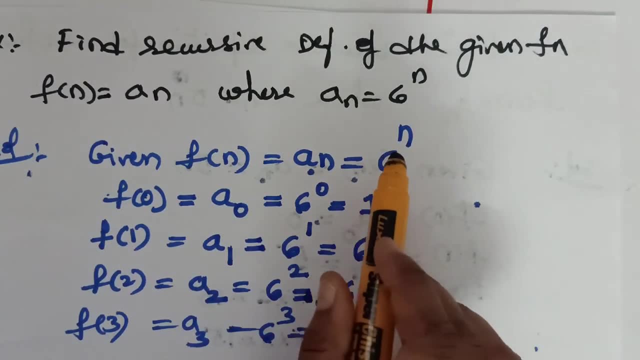 recursive definition. therefore, it is the recursive definition of the function f of n is equal to a n, where a n is equal to 6 power n. similarly,